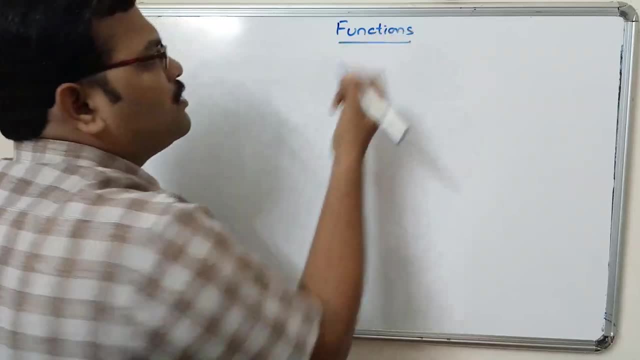 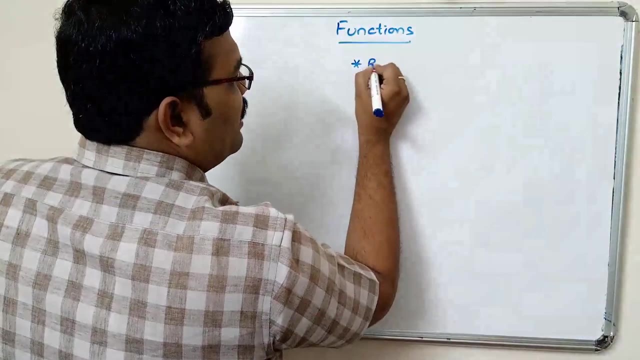 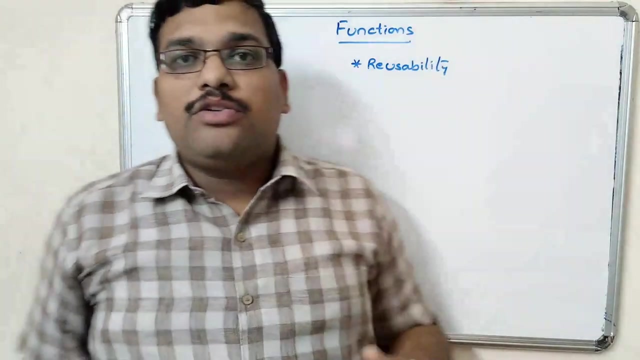 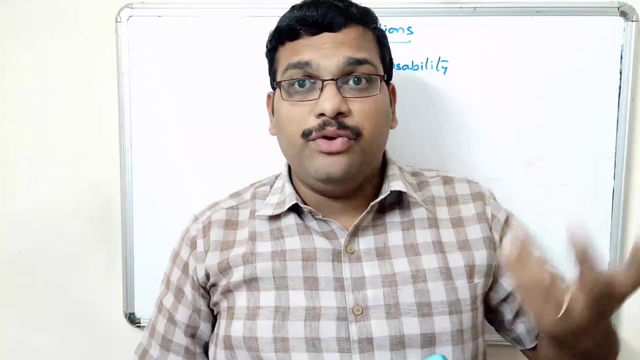 So the major usage of writing these functions is reusability. in order to achieve the reusability, So reusability means once we write any function, that function can be called a number of times. That means we can use that function in many programs. 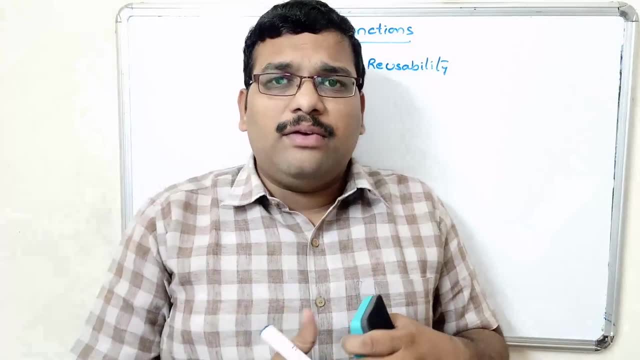 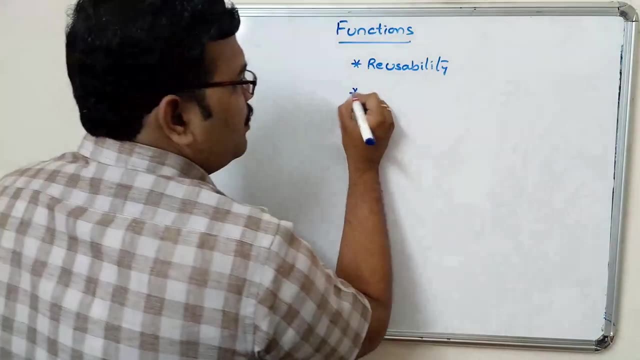 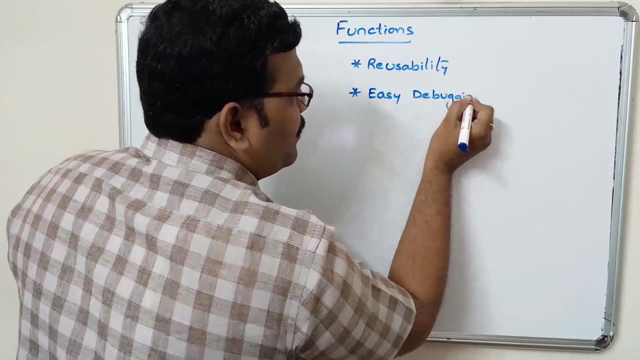 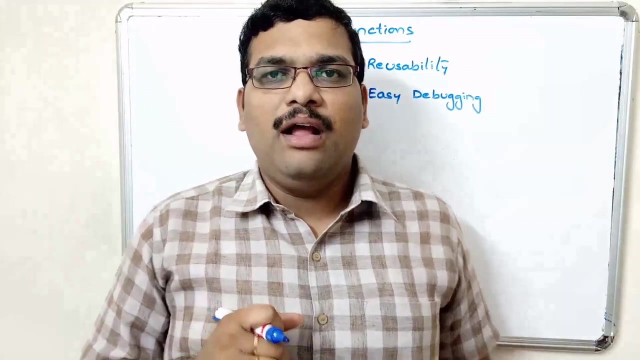 So, in order to rewrite any function, any logic, we can write a single generalized function and we can make use that function number of times and also easy debugging. that means the finding and rectifying the errors will be easy for the user if we write these functions. so in the absence of functions, if 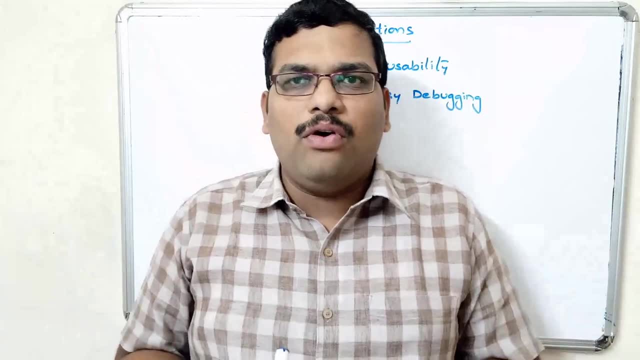 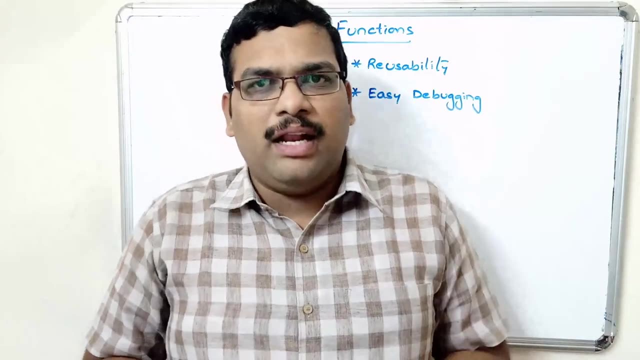 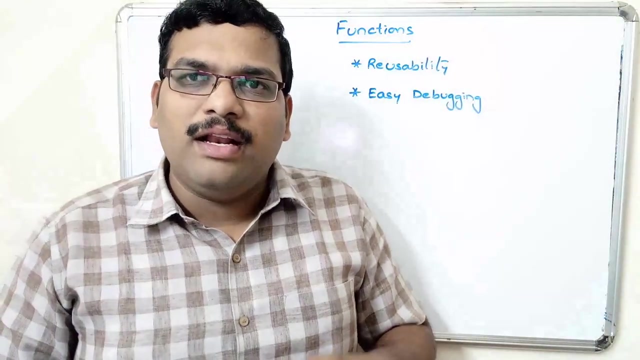 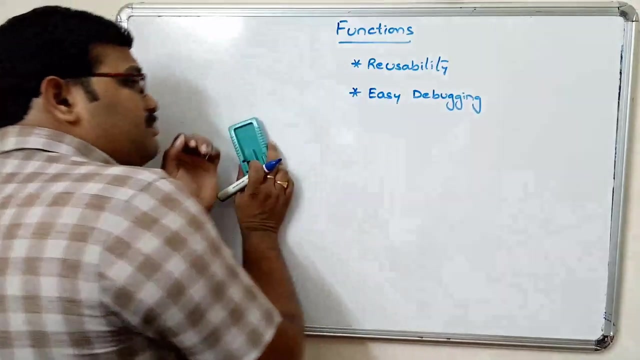 any program needs more lines of code or more complex logic, then it would be difficult to find the errors. in case of logical error it is somewhat difficult to find the logical errors right. so if that can be written in functions then automatically this debugging process will be easier for the user right. so the major reasons to writing the functions. 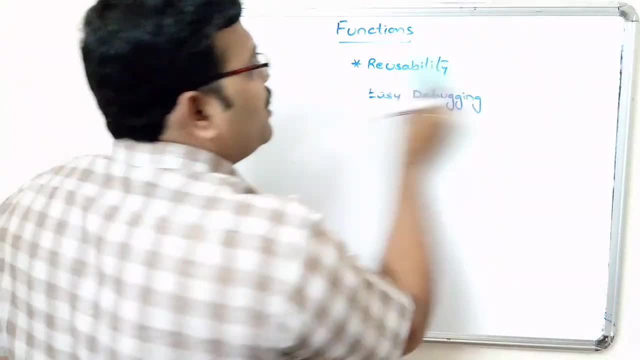 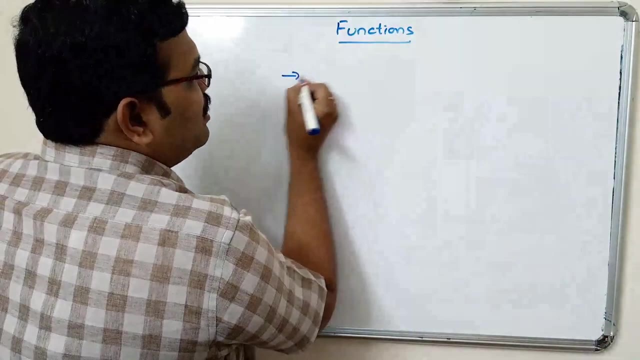 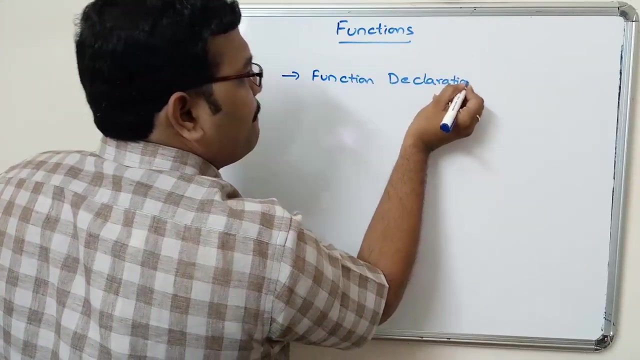 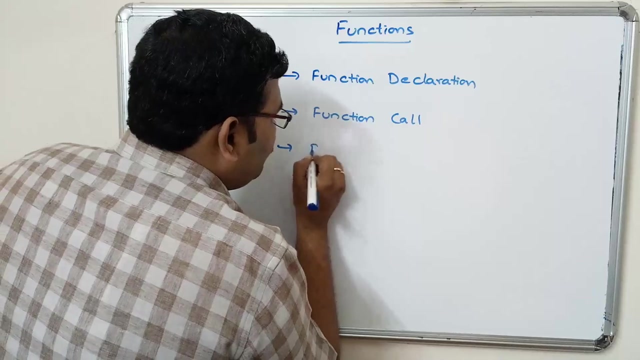 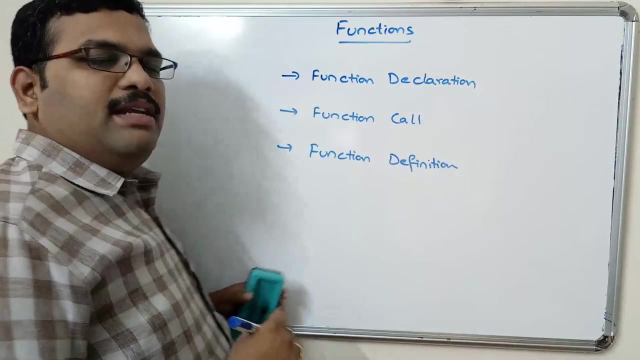 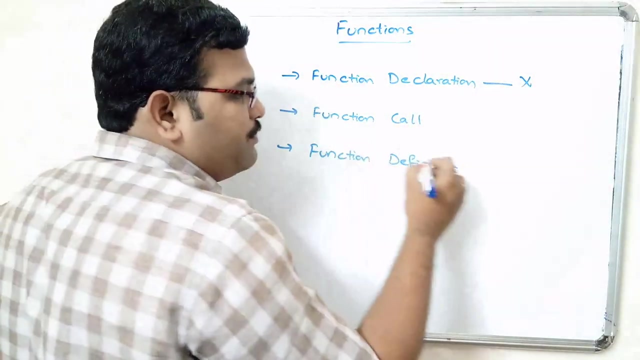 is reusability and for easy debugging now, so similar to the variable in C language we have seen the function declaration, next function call, next function definition. so this we have seen in C programming. so here we can avoid this declaration because so first we have to start writing the function. 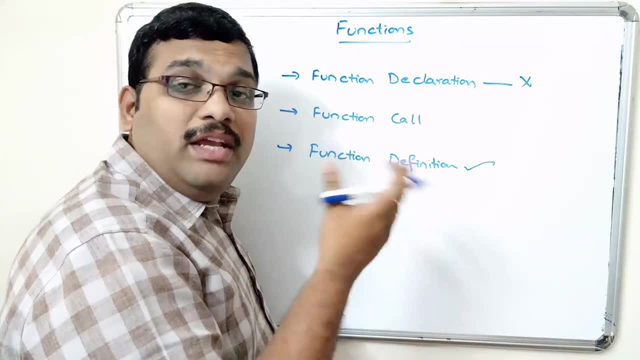 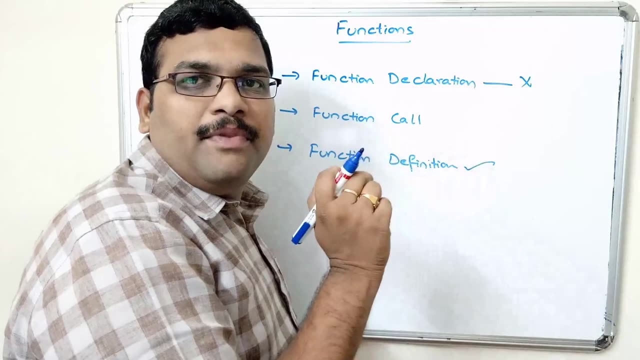 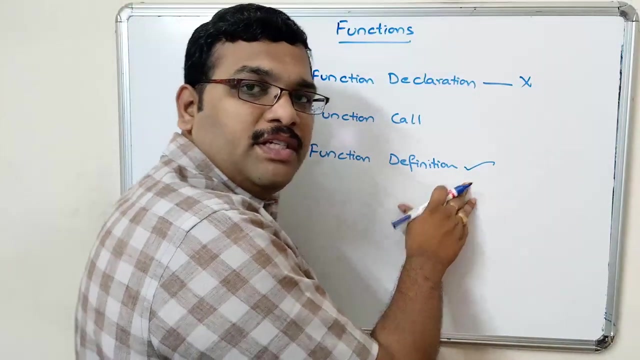 definition and then we will write the actual program. so here we are not writing the many main functions I am just mentioning as a actual program. right? instead of using the main function I am, I am using the actual program. so first we have to write the function definition and 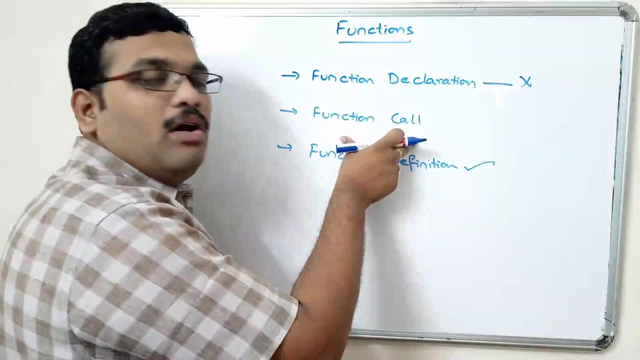 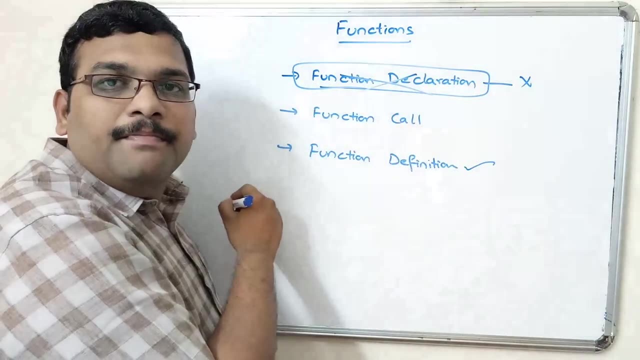 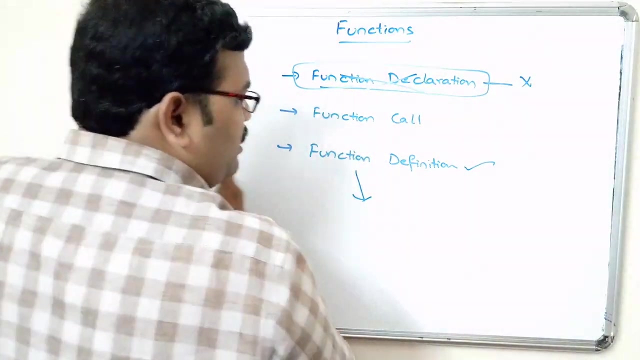 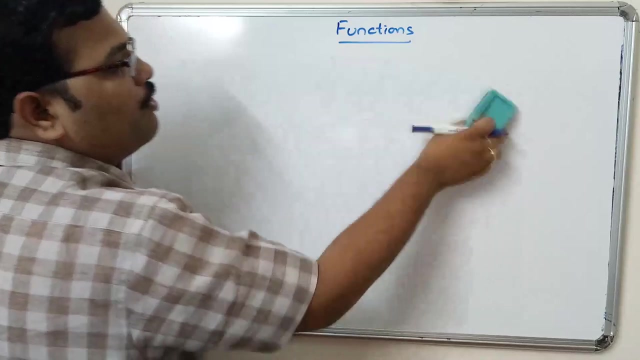 then we have to write the actual program where this function call is inclusive programming, right home. So that's why this function declaration is not needed in Python programming, right? so how this function definition can be done so here in the function definition. so let us see that. so what are the parameters involved in the function definition? 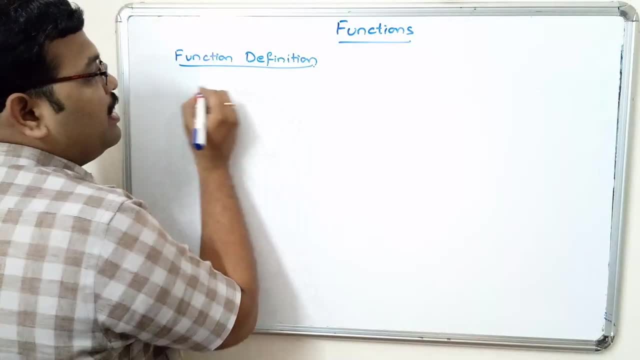 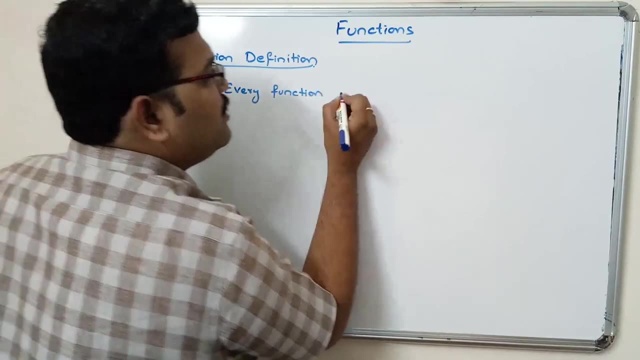 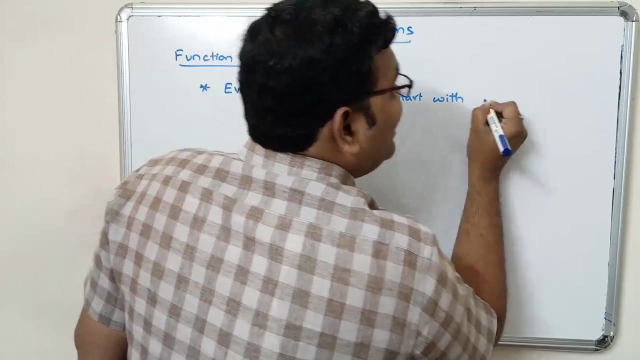 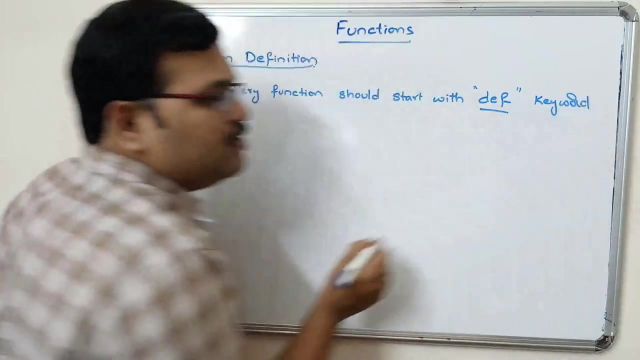 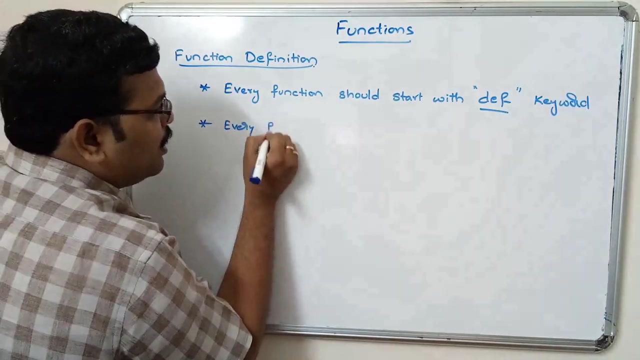 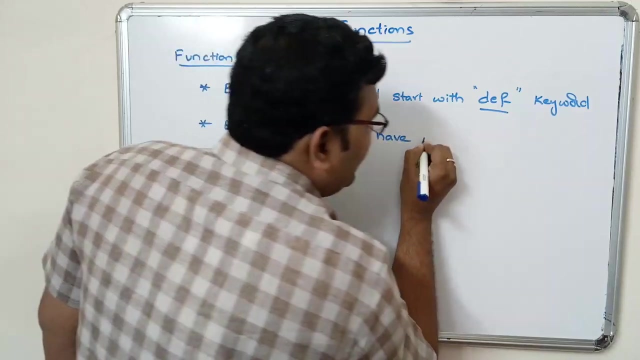 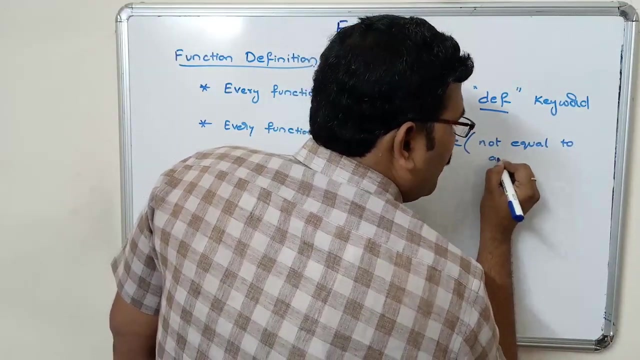 a function definition. so first one is: every function should start with DEF keyword. so we are having the D E F keyword, so all the function functions should solve start with D F keyword. then every function should have a name. should have a name not equal to any keyword, so the same. 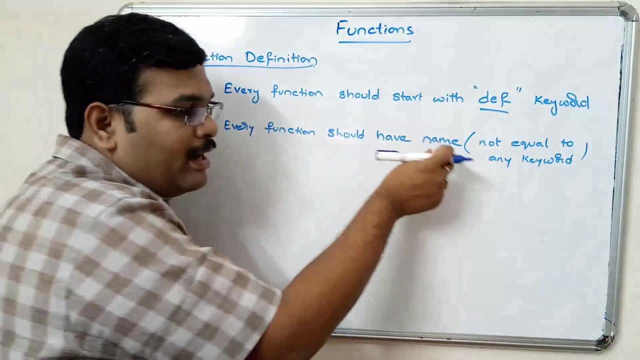 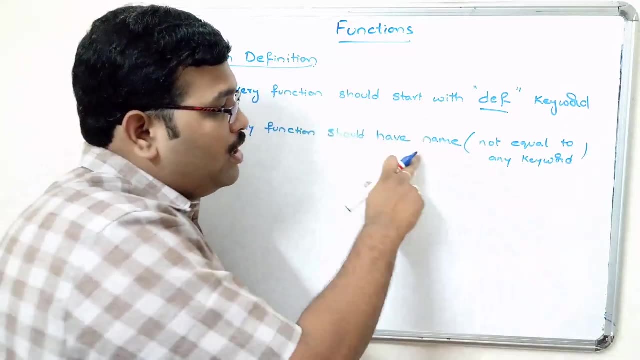 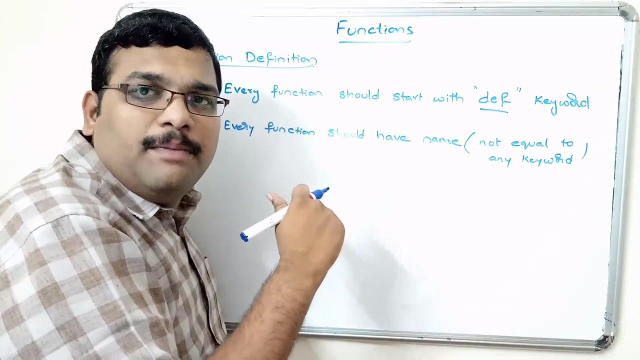 rules we have applied in C language right. so we have to give one name, specific name, to the function, because this is a user defined function, so the user is writing the function. so we should give some name and that should not be equal to any one of the keyword. so we have discussed the keywords in the 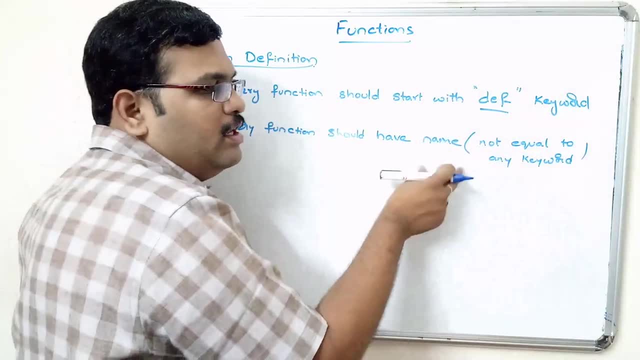 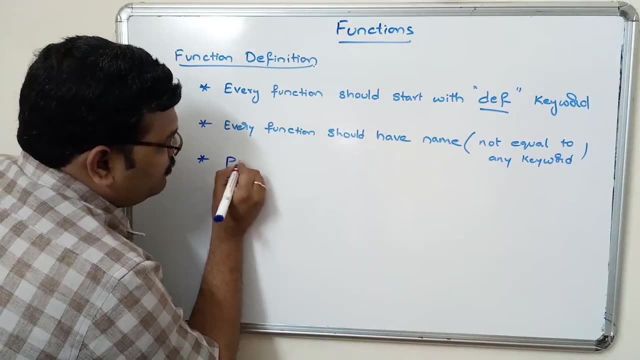 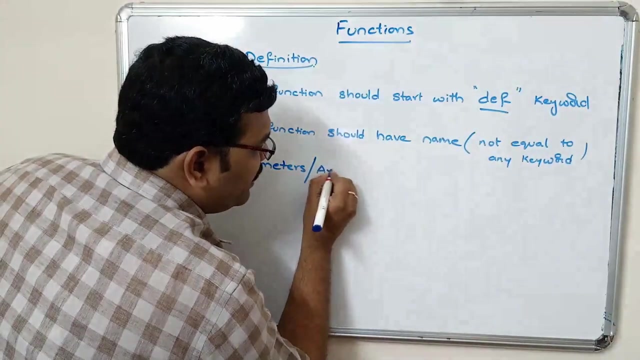 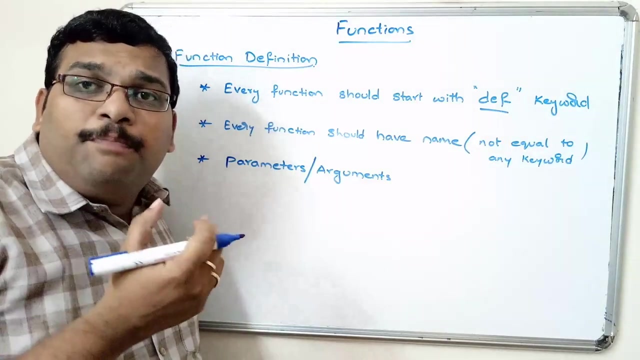 previous session, so just go through the keywords session. so this name should not match it any one of the keyword. next one is parameters, or we can call them as arguments. so parameters or arguments are nothing but the inputs given to that particular. you're a different function, so this is an optional. 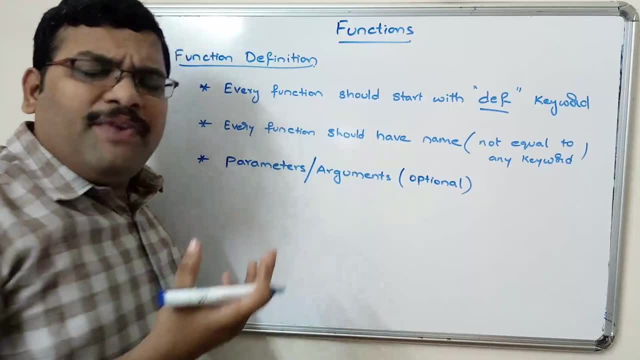 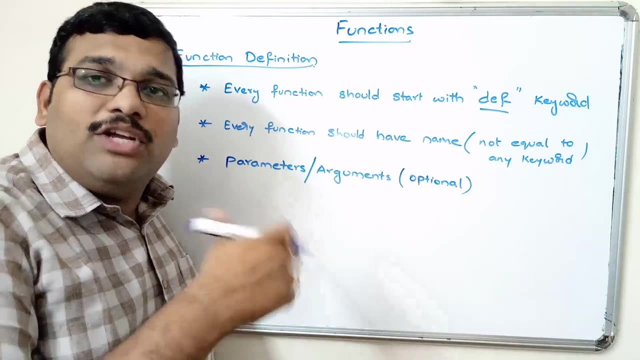 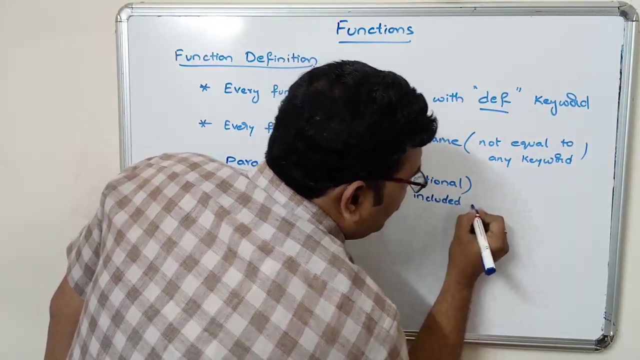 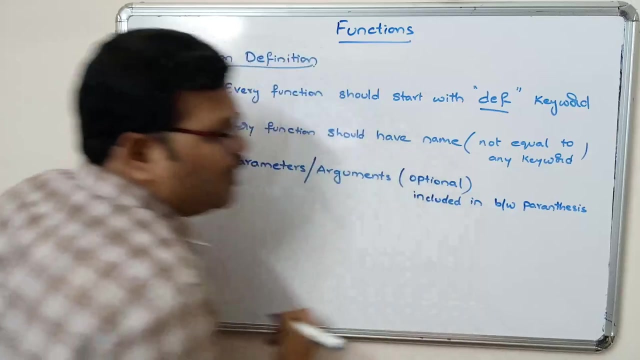 this is an optional, so every function may have the parameters or arguments or may not have. the parameters are on that, so you can have a zero or more parameters or- and these should be included in between right. so first we have to write the definition- I mean DEF keyword- then we 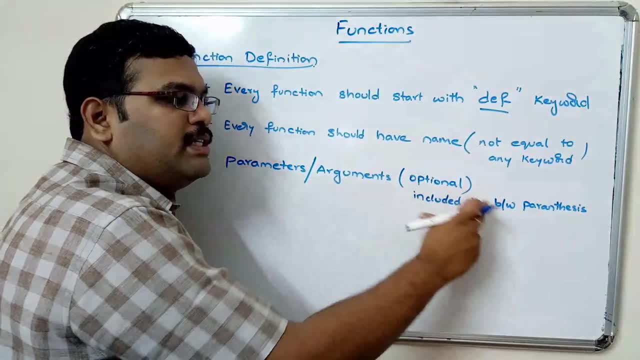 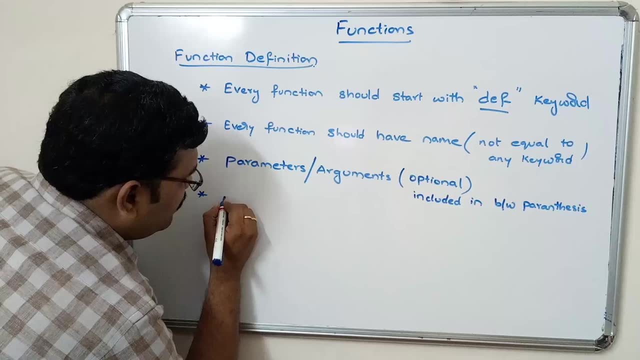 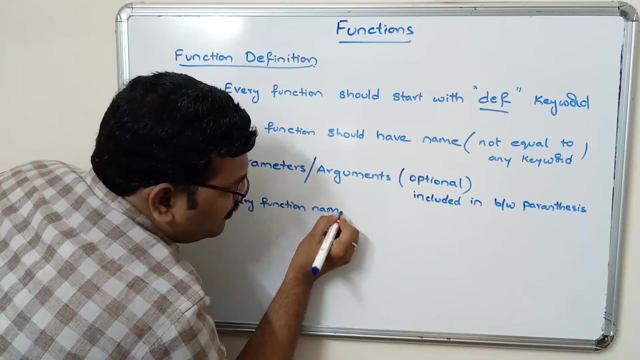 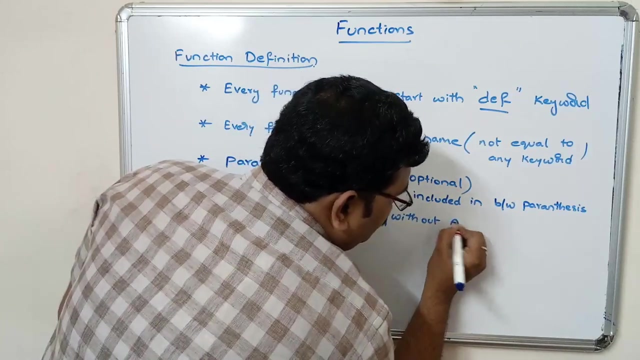 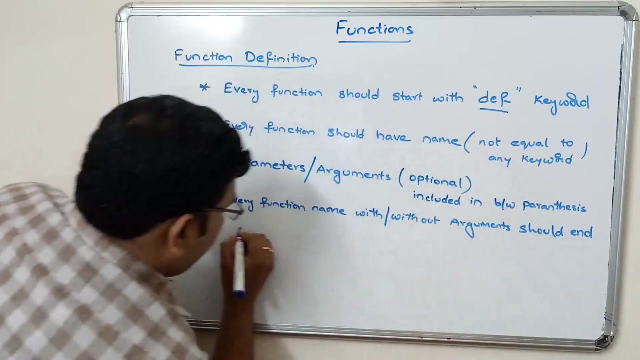 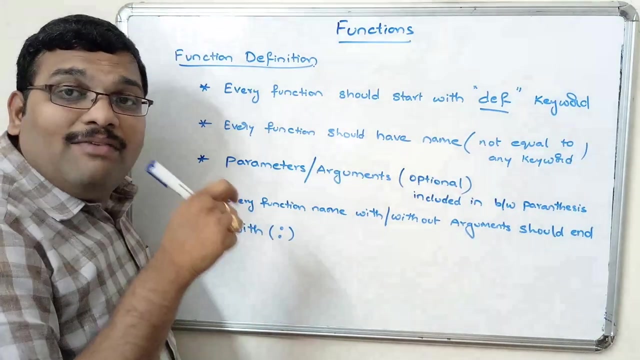 have to write the name, and then we have to write the parameters or arguments in between the parentheses. right, this one is an optional. next fourth one: every function name, with or without arguments, should end with colon. so because in our C language we are not using the curly braces. so instead of representing the block of 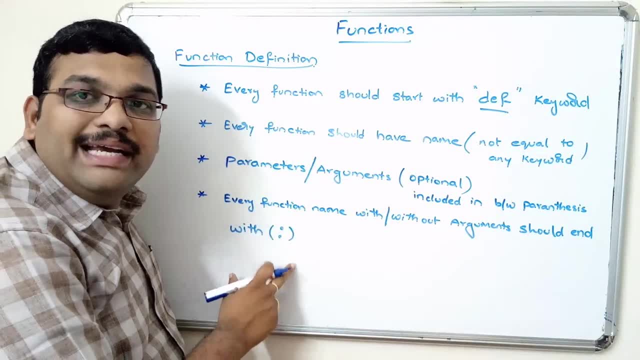 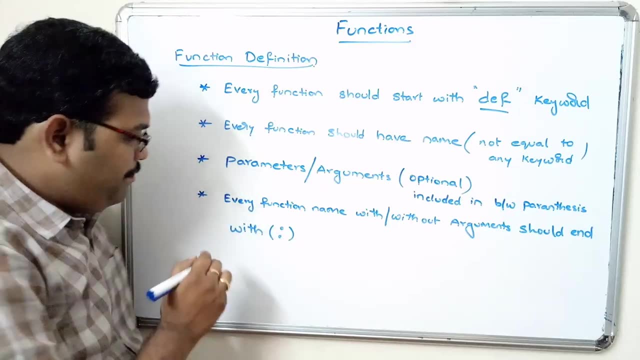 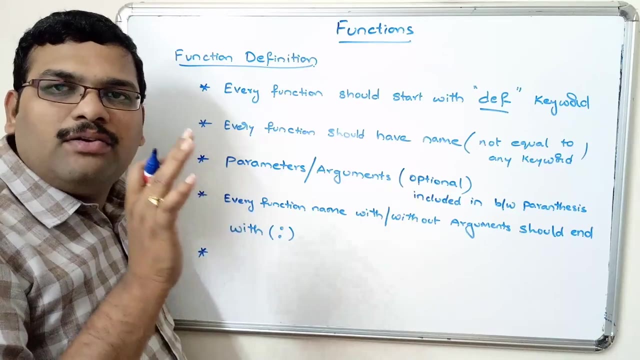 words. we are not using the curly braces, so instead of representing the block of statements, that can be done only by using the indentation. so here to achieve the indentation we have to use this column right next, every function will be having some return, so that return can be any value return or an empty return. so 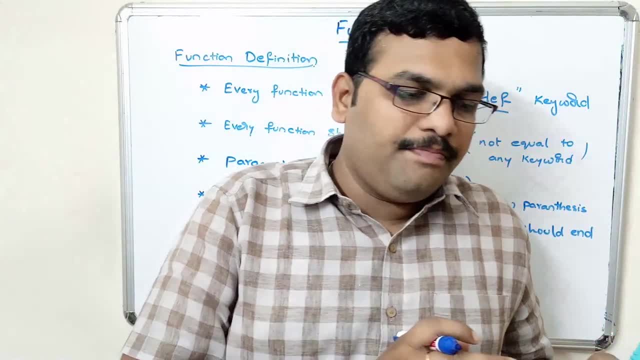 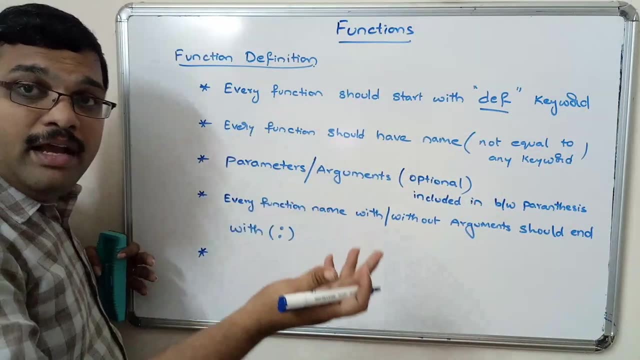 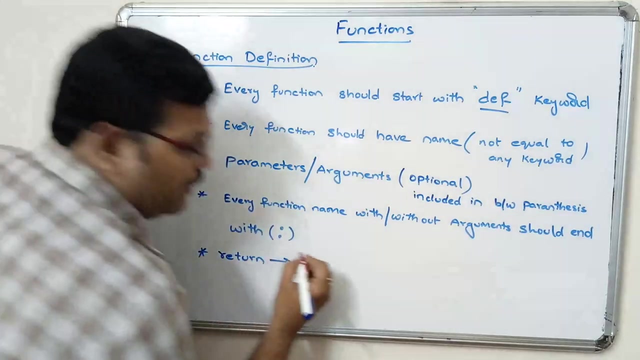 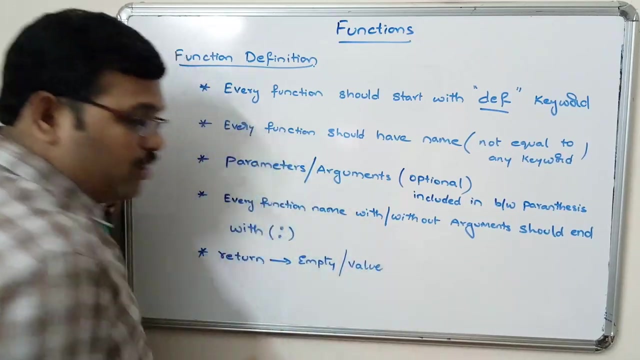 finally, the control will return to its calling function. so every function will return to its calling function. that may be an empty return or any value return right. so return right. it can be empty or a value return. so in C language, every function will return only a single. 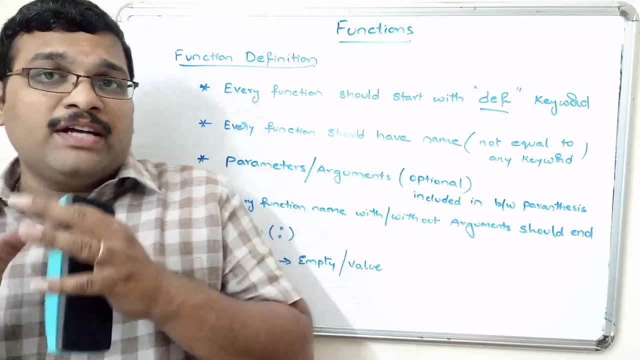 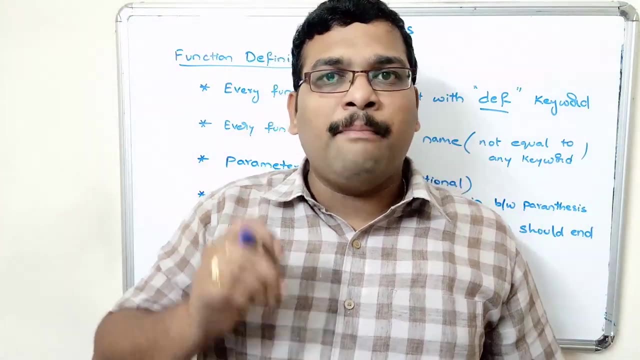 value. but it cannot. well, that means a function cannot return the multiple values. but here in Python programming so function can return a multiple values. but here in Python programming so function can return a multiple values to the calling function. that is done only by using tuples in the form of. 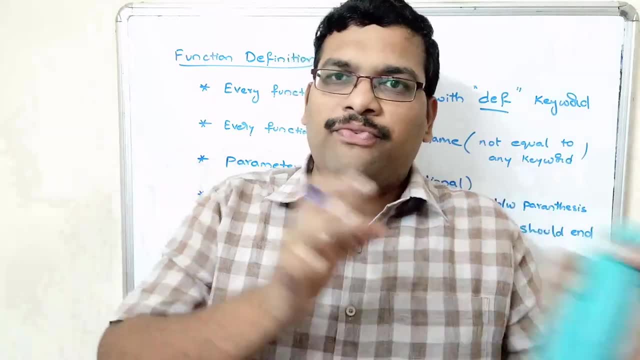 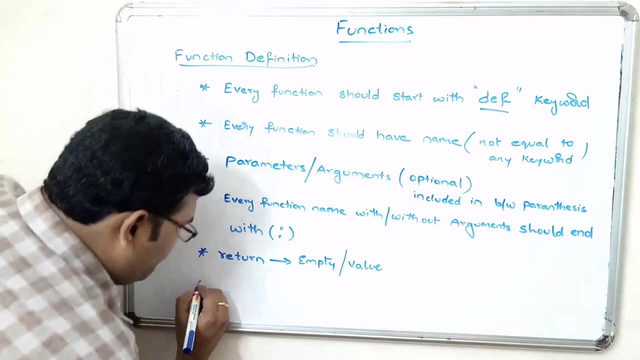 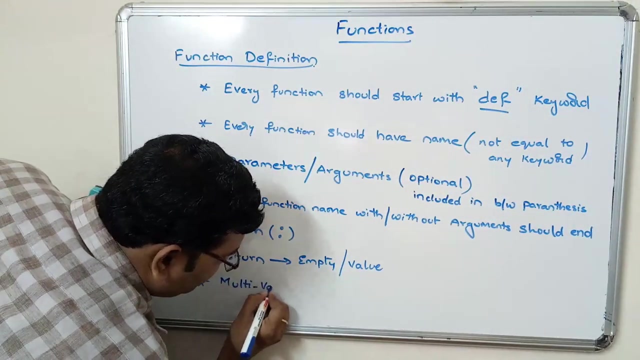 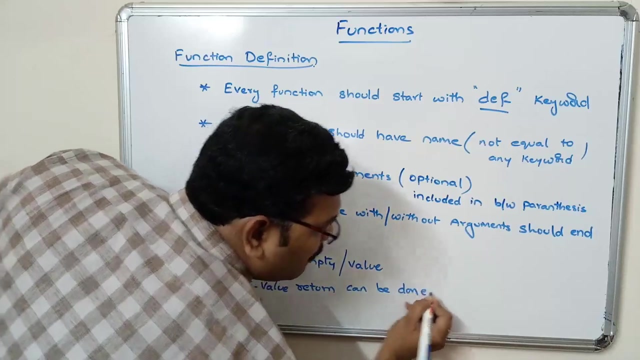 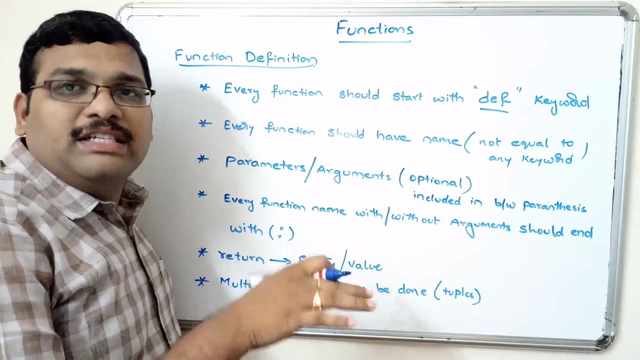 tuples, right. so in case of returning the multiple values, that will be done only by using tuples. so here the multiple return can be accepted. multi value return can be done using tuples, right. so these are some important points while writing the function. function definition, right? so first it should start with the 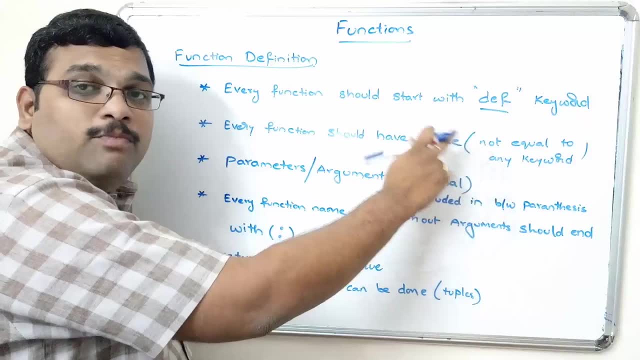 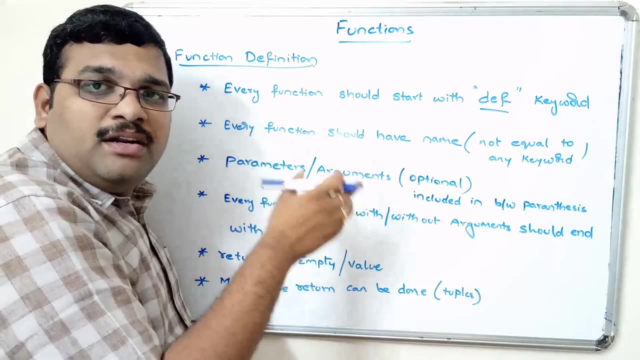 DEF keyword. next, it should have some name, which is which does not match with any one of the keywords, and then we have to write the parameters. that means inputs to the function. that may be an option. that may be an option. that may not be an option. that may be an option. 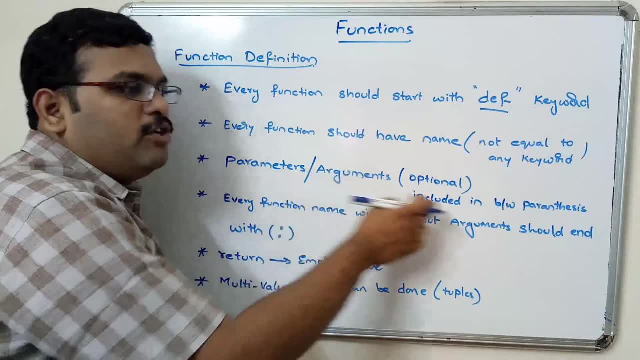 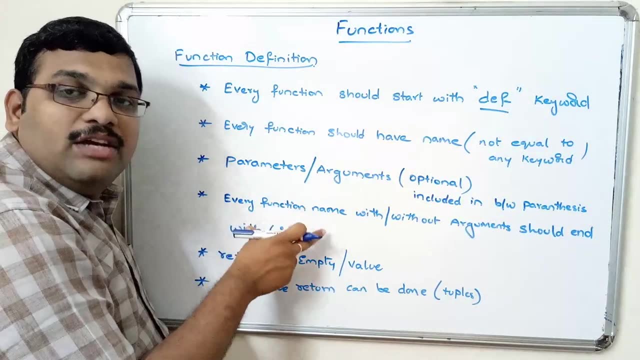 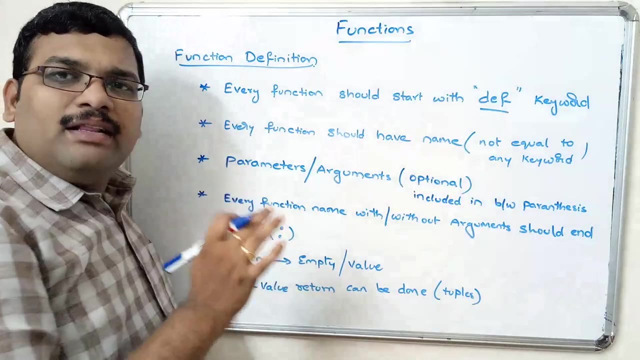 thing, and these parameters or arguments must be included in between the balances and after the balance is: every function should end with colon, so this gives the indentation that means a block of which represents the block of statements. next, every function will return the control to its parent function. 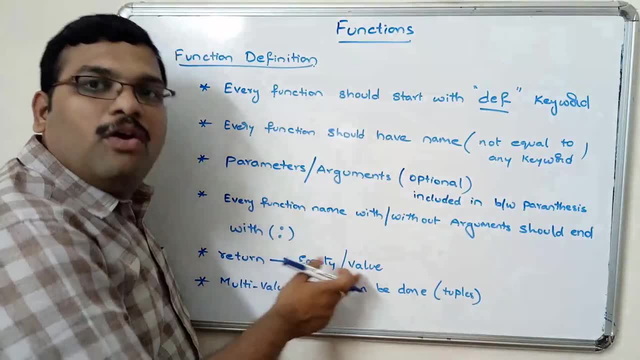 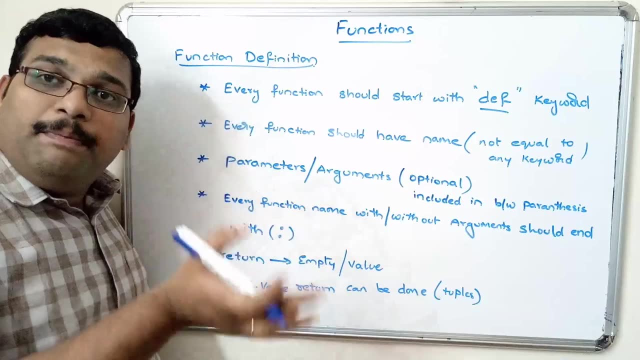 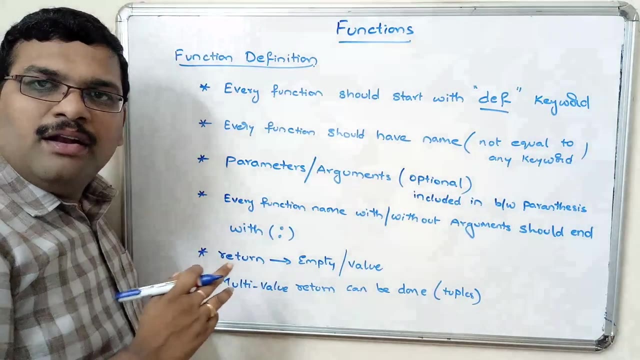 calling function so that, may that can be an empty return or a value return, here the multi value return can be done. that means one function can return multiple values, and that can be done only by using tuples. so how we understood this function definition. right now let us move on to the function call. 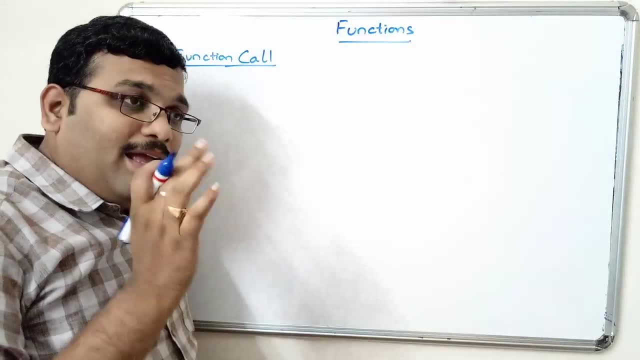 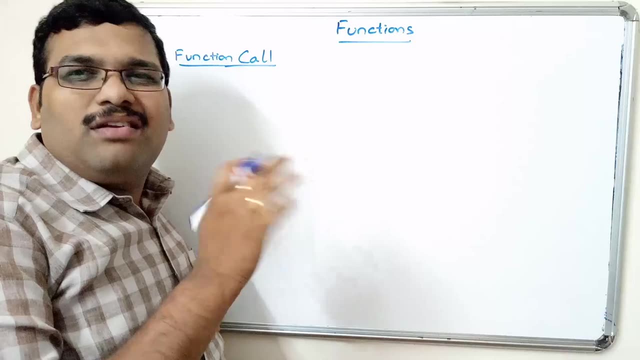 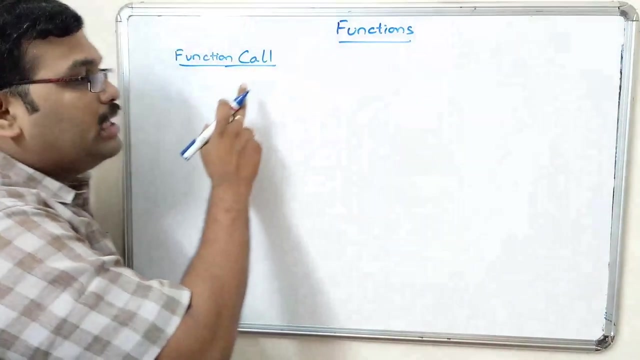 function call. so, as we discussed in the C programming, we have to write this function call in the main function or some parent function that is called as calling function, right? so here also, while writing the program, we have to declare this function call and by whatever control executes this function call automatically, the control moves to the 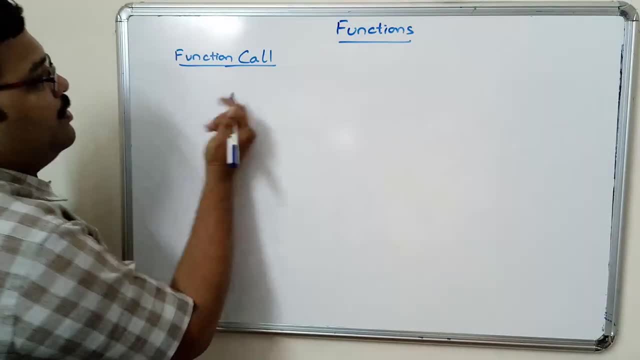 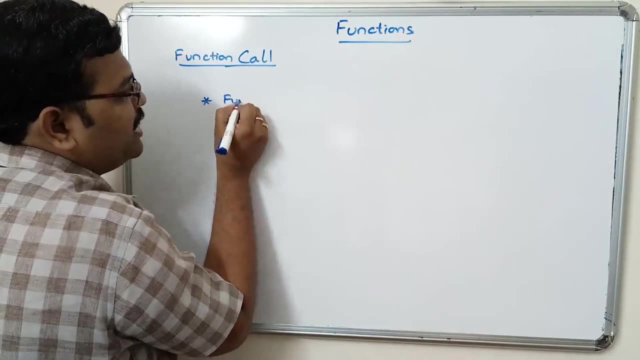 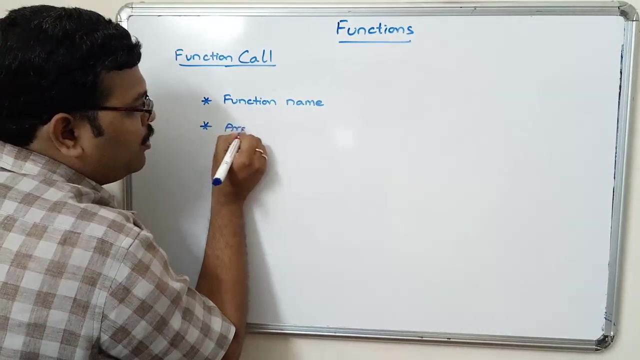 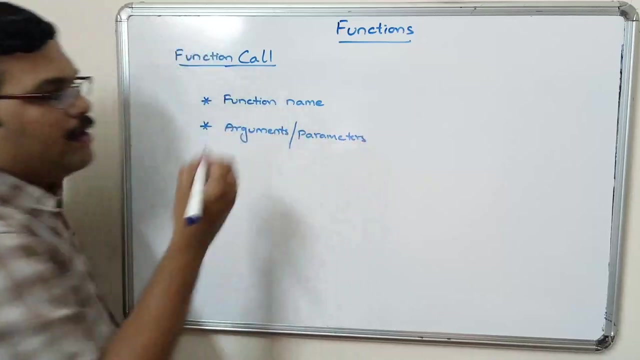 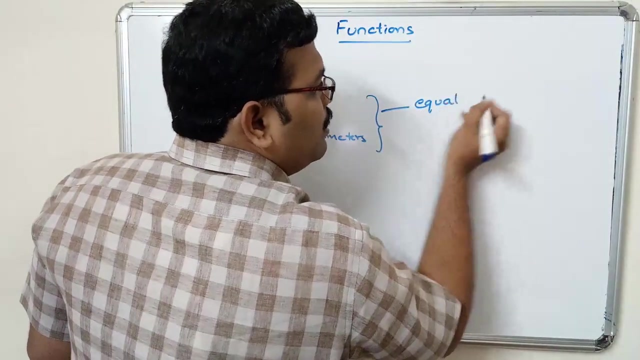 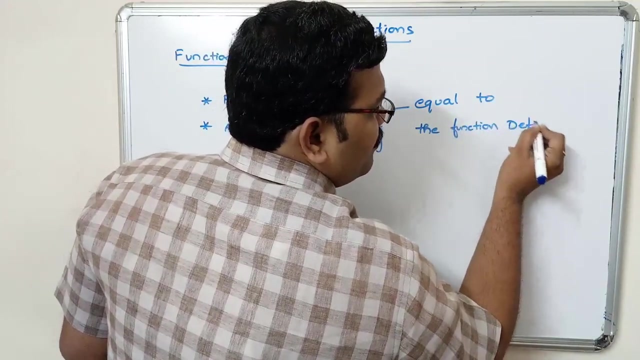 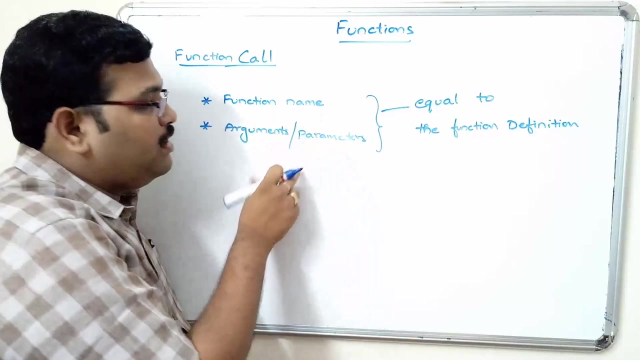 function definition, right C. so here the function call also have function name, here also the function name, arguments or parameters. the only thing is this: function name and parameters should be equal to the function definition right. so this one, the same function name should be written in function definition and the same. 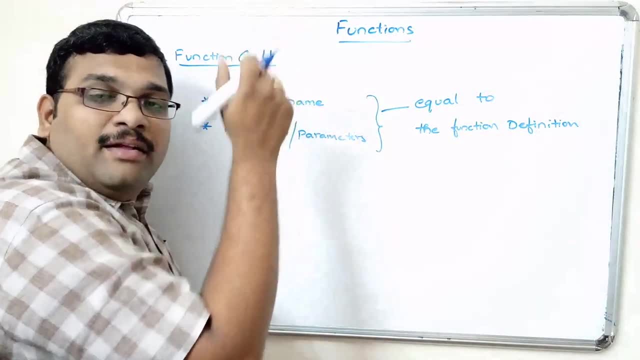 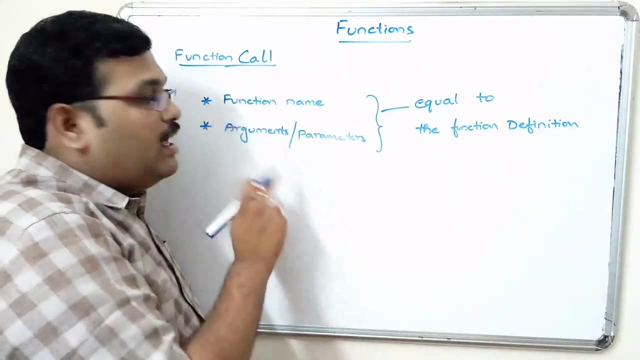 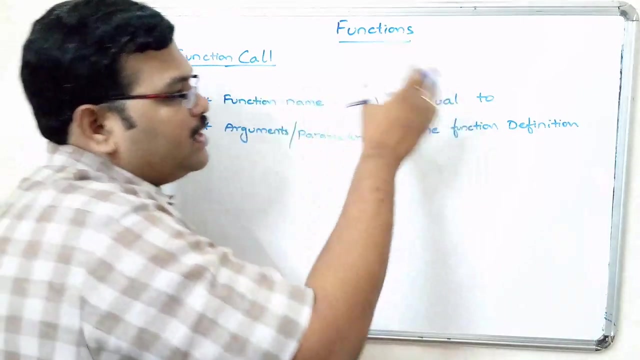 number of arguments or parameters should be written in function definition right. the number of arguments should be equal in both the function call and function definition and the function name should also be equal in both function name and function definition right. and this function, this function call, will be. 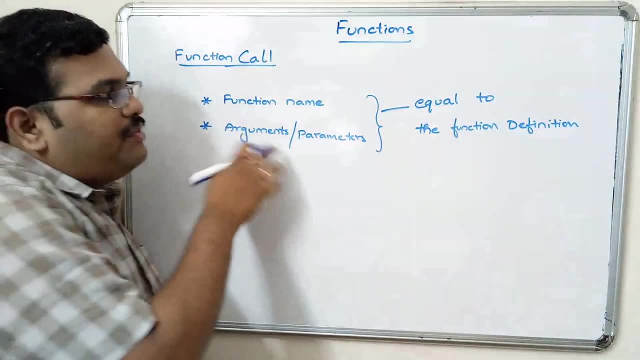 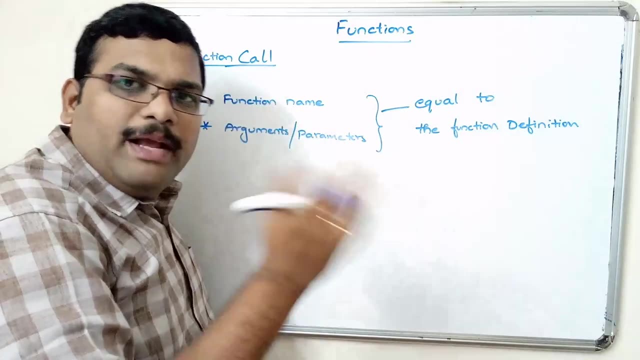 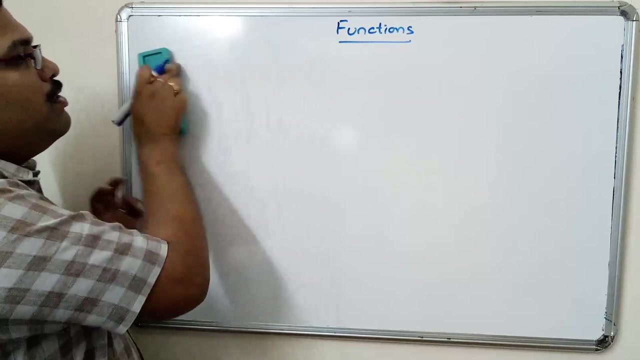 written and whenever the control comes, execute this function call. automatically the function definition will be executed. so let us see an example so that this you the typical be clarify right. as I said before, here there is no question of function declaration, because the function definition will always starts. 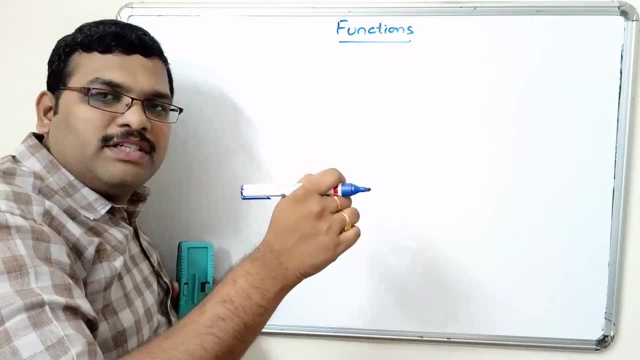 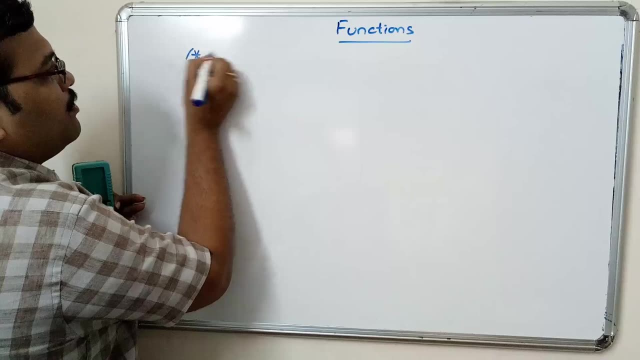 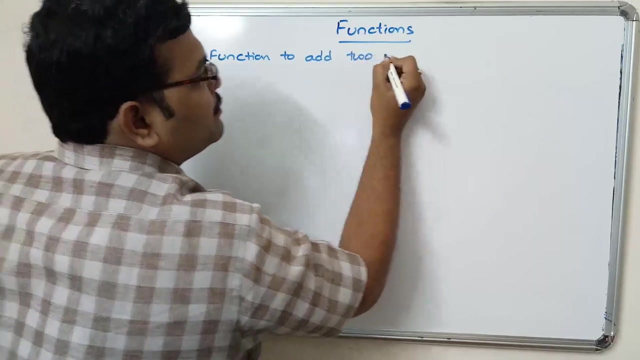 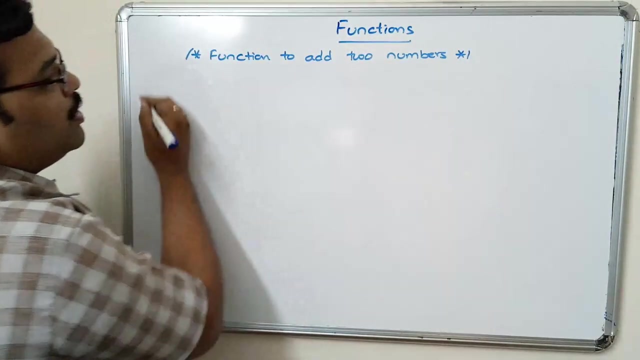 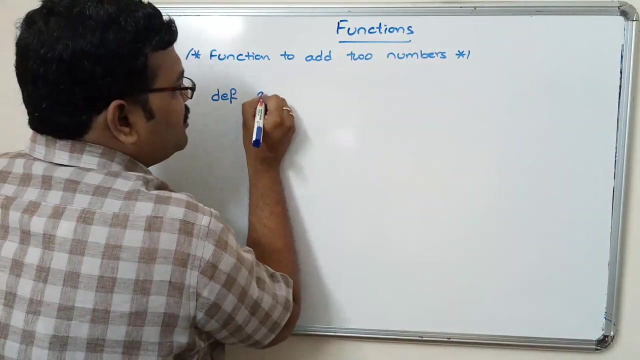 at the beginning. so first we have to write the function definition, then only we have right the actual program see: function to add two numbers. function to add two numbers. so first we have to write the function definition, right. so function definition, we have to write def, some add, write the parameters, some a, comma, b. 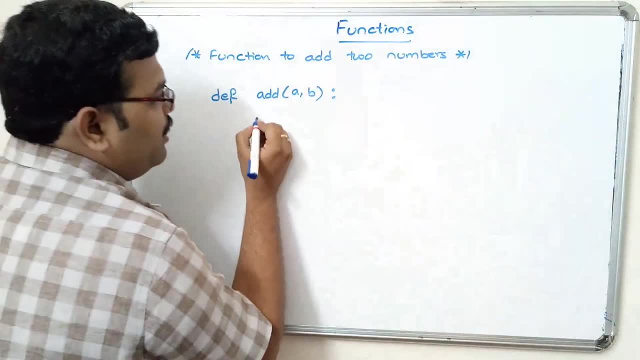 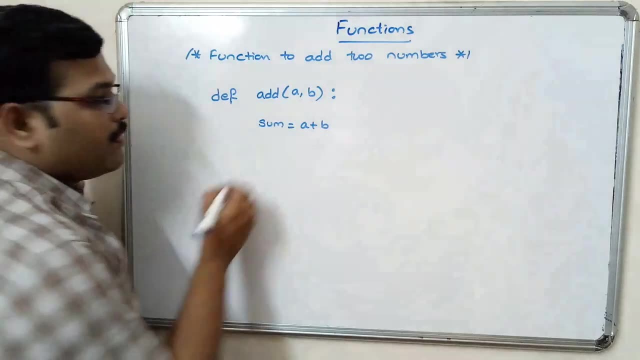 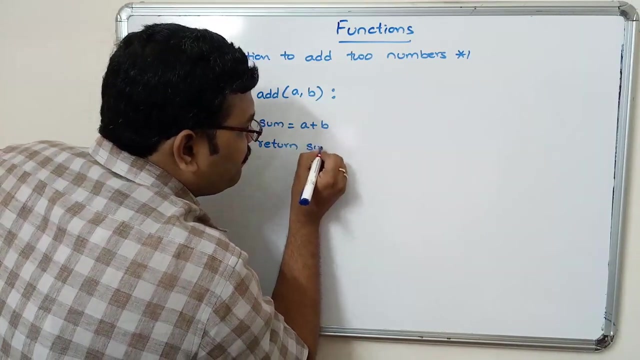 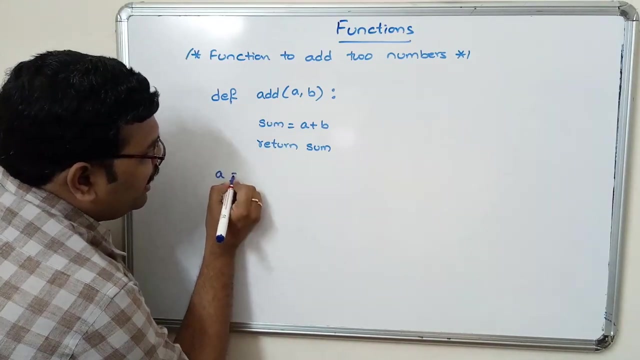 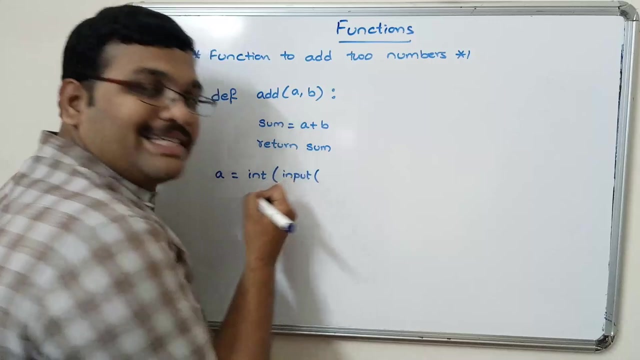 use the column because this represents the indentation. now here we can write: sum is equal to a plus b and next we have to write return or directly we can write a plus b in return, right return sum. right now write the actual program: a is equal to typecast because the input function always take the string. 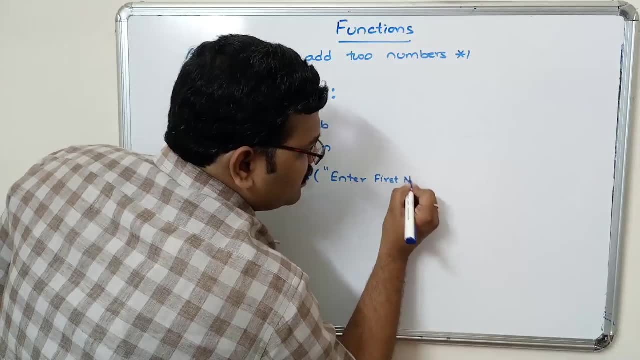 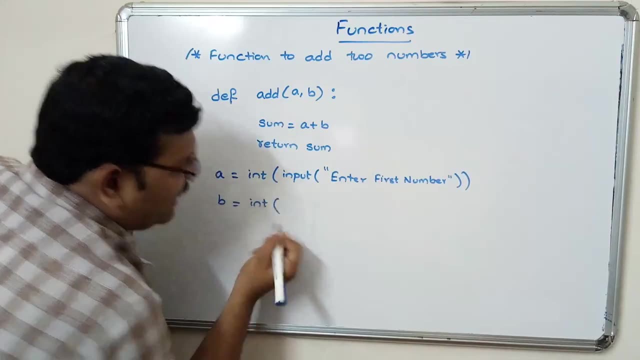 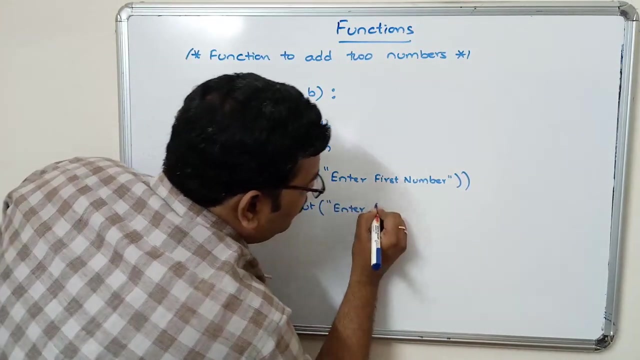 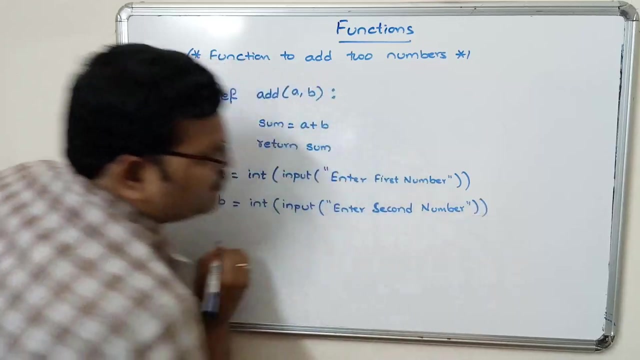 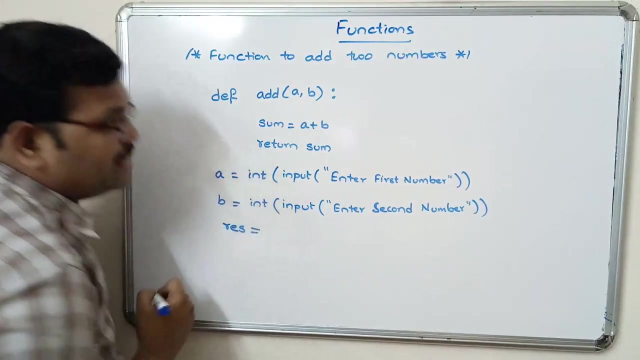 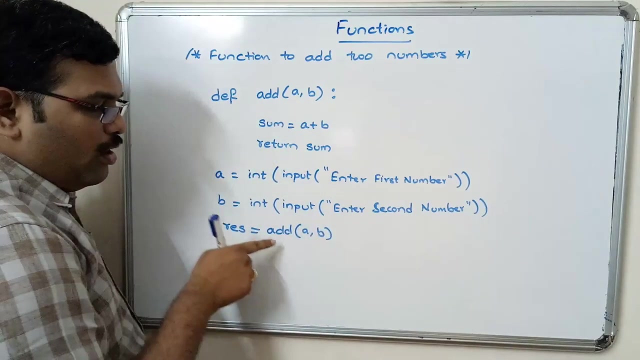 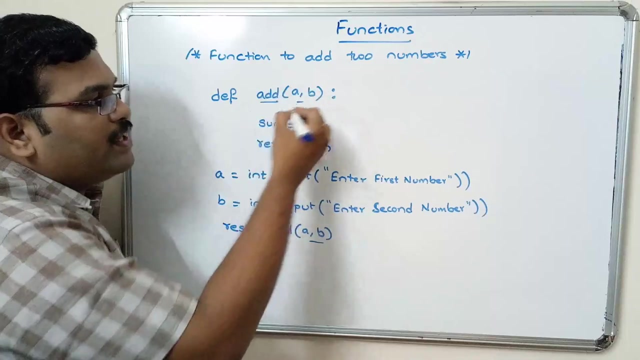 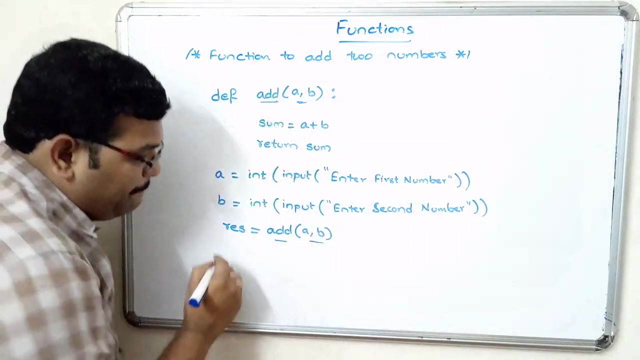 enter first number. next b is equal to. so reading the two values: input values: input: enter second number. now write the function column: result is equal to add of a comma b. so this is a function call. here see the function name. in both the function definitions are equal. the number of parameters in both the function definition and function call are equal. so here we are passing two arguments, here we are calling the two arguments right now. print the result. print.